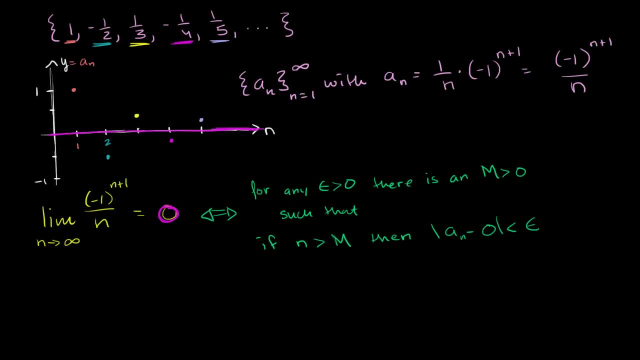 We're saying: give us an epsilon around zero. So let's say that this right over here is zero plus epsilon. That is zero plus epsilon. The way I've drawn it here, it looks like epsilon would be .5.. This would be zero minus epsilon. 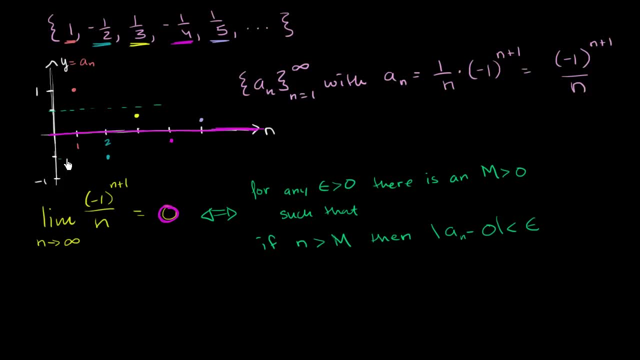 Let me make it a little bit neater. So this would be zero minus epsilon. So this is negative epsilon zero minus epsilon. zero plus epsilon. Our limit, in this case our claim of a limit, is zero. Now this is saying for any epsilon. 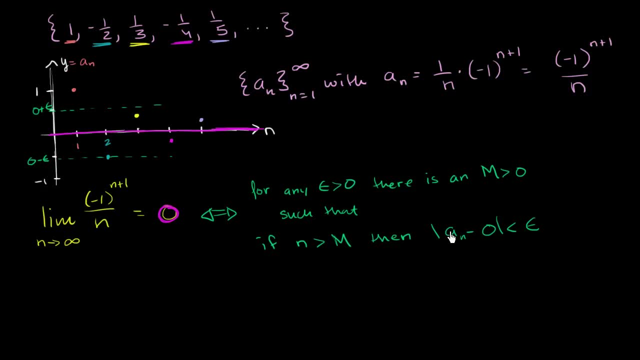 we need to find an M such that if N is greater than M, the distance between our sequence and our limit is going to be less than epsilon. So if the distance between our sequence and our limit is less than epsilon, that means that the value of our sequence for a given N 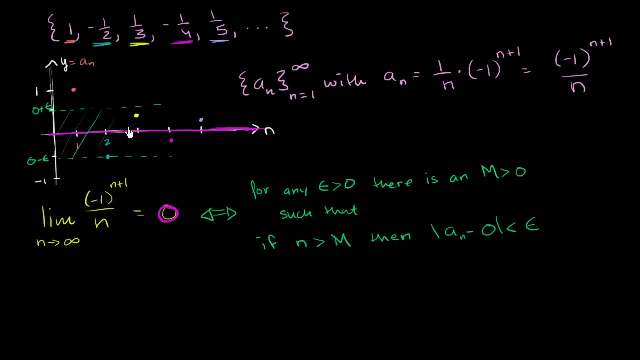 is going to be within these two bounds. It's gotta be in this range right over here that I'm shading above a certain N, So if I pick an N right over here, it looks like anything larger than that is going to be the case that we're going to be. 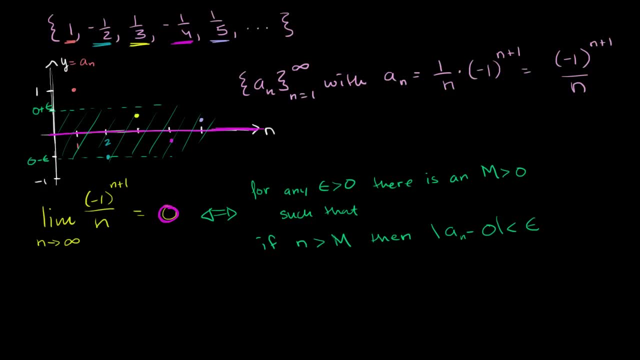 within those bounds. But how do we prove it? Well, let's just think about what needs to happen for this to be true. So what needs to happen for a sub N minus zero- the absolute value of a sub N minus zero, what needs to be true for this to be less than epsilon? 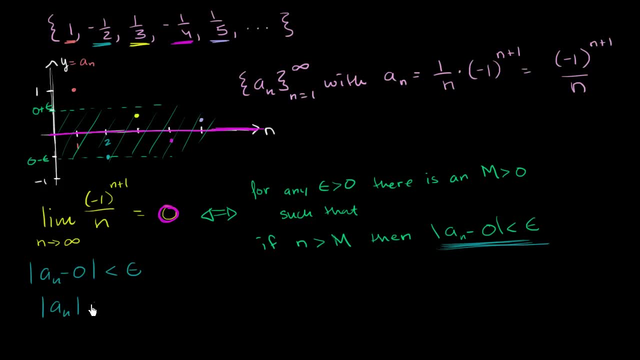 Well, this is another way of saying that the absolute value of a sub N has to be less than epsilon, And a sub N is just this business right here. so it's another way of saying that the absolute value, the absolute value of a sub N, is less than epsilon. 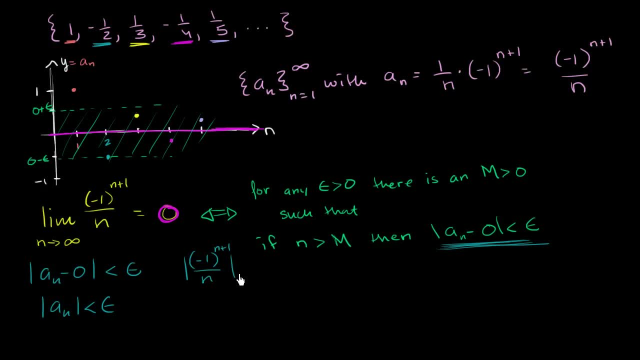 So the absolute value of negative one to the N plus one over N has to be less than epsilon, which is another way of saying, because this negative one to the N plus one, this numerator, just swaps us between a negative and a positive version of one over N. 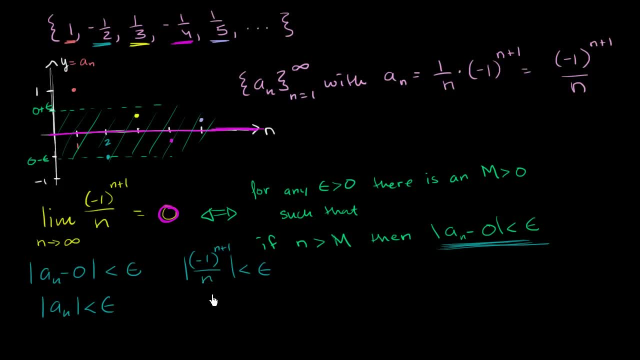 But if you take the absolute value of it, this is always just going to be positive. So this is the same thing as one over N. as the absolute value of one over N has to be less than epsilon, Now N is always going to be positive. 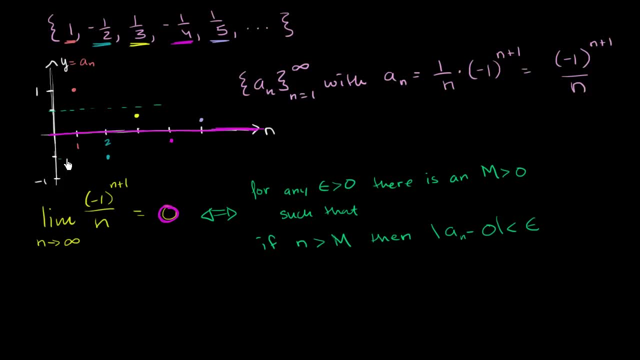 Let me make it a little bit neater. So this would be zero minus epsilon. So this is negative epsilon zero minus epsilon. zero plus epsilon. Our limit, in this case our claim of a limit, is zero. Now this is saying for any epsilon. 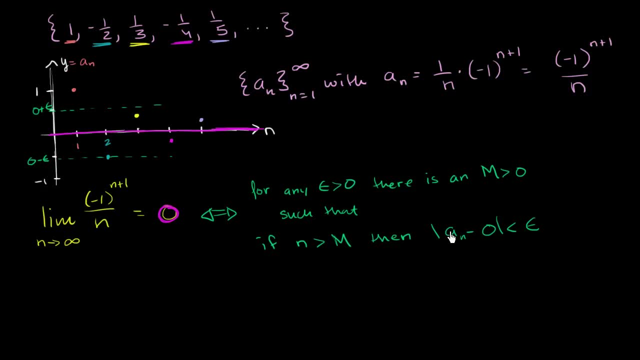 we need to find an M such that if N is greater than M, the distance between our sequence and our limit is going to be less than epsilon. So if the distance between our sequence and our limit is less than epsilon, that means that the value of our sequence for a given N 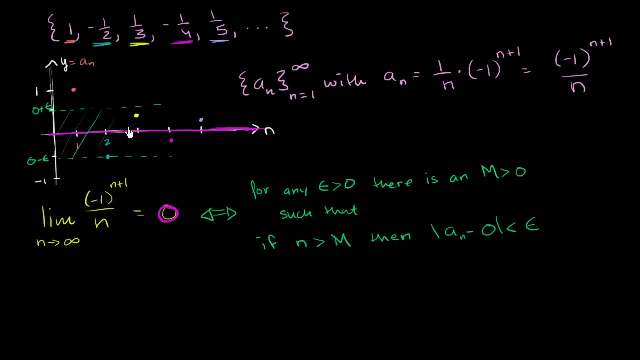 is going to be within these two bounds. It's gotta be in this range right over here that I'm shading above a certain N, So if I pick an N right over here, it looks like anything larger than that is going to be the case that we're going to be. 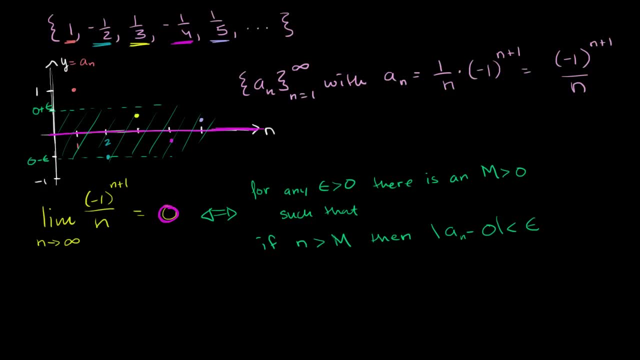 within those bounds. But how do we prove it? Well, let's just think about what needs to happen for this to be true. So what needs to happen for a sub N minus zero- the absolute value of a sub N minus zero, what needs to be true for this to be less than epsilon? 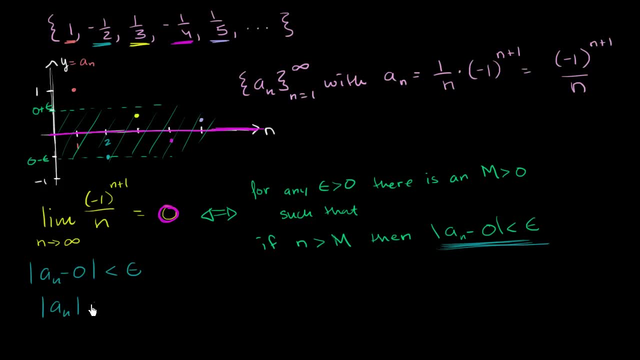 Well, this is another way of saying that the absolute value of a sub N has to be less than epsilon, And a sub N is just this business right here. so it's another way of saying that the absolute value, the absolute value of a sub N, is less than epsilon. 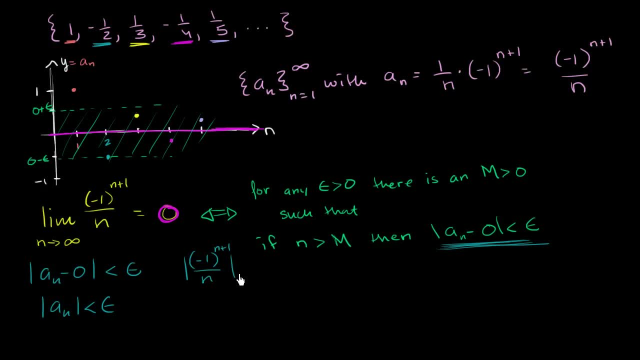 So the absolute value of negative one to the N plus one over N has to be less than epsilon, which is another way of saying, because this negative one to the N plus one, this numerator, just swaps us between a negative and a positive version of one over N. 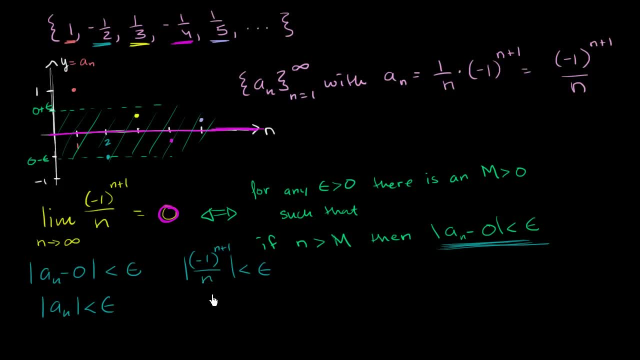 But if you take the absolute value of it, this is always just going to be positive. So this is the same thing as one over N. as the absolute value of one over N has to be less than epsilon, Now N is always going to be positive. 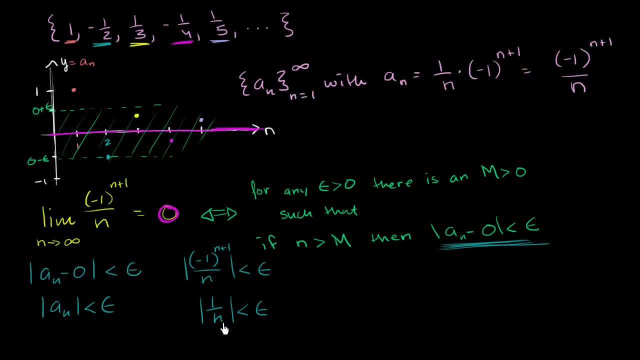 N starts at one and goes to infinity, So this value is always going to be positive. So this is saying the same thing: that one over N has to be less than epsilon in order for this stuff to be true. And now we can take the reciprocal of both sides. 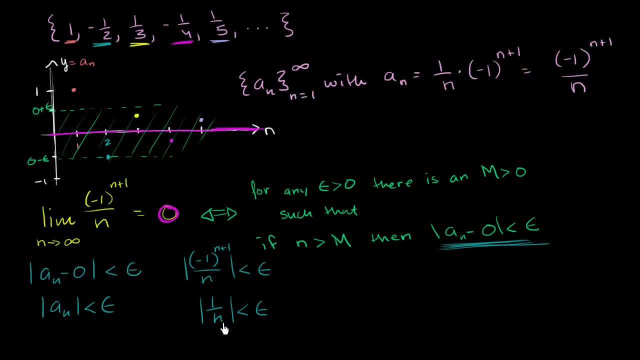 N starts at one and goes to infinity, So this value is always going to be positive. So this is saying the same thing: that one over N has to be less than epsilon in order for this stuff to be true. And now we can take the reciprocal of both sides. 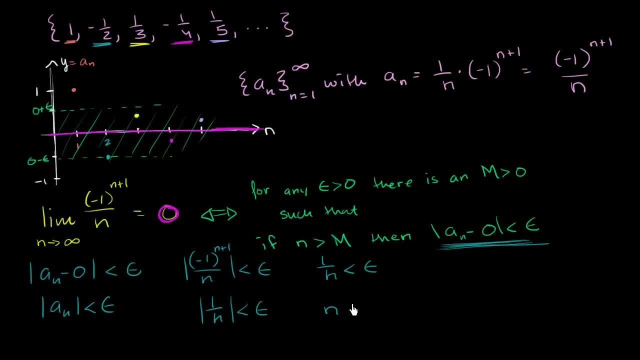 And if you take the reciprocal of both sides of an inequality, you would have that N. if you take the reciprocal of both sides of an inequality, you swap the inequality. So this is: for this to be true, N has to be greater than one over epsilon. 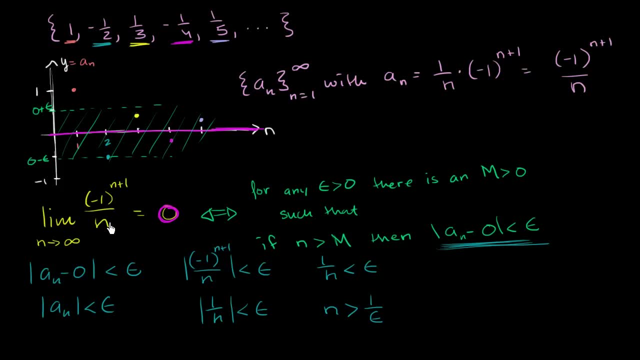 And we essentially have proven it now. So now we've said: look for this particular sequence, you give me any epsilon and I'm going to set M to be one over epsilon, Because if N is greater than M, which is one over epsilon. 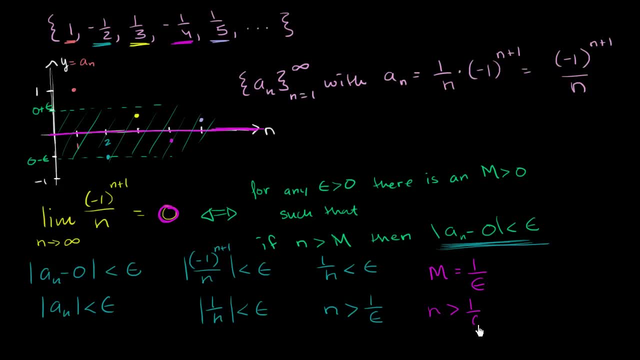 if N is greater than one over epsilon, then we know that this, right over here, is going to be true. That is going to be true. So the limit does definitely exist. And so, over here, for this particular epsilon, it looks like we picked 0.5, or 1 half as our epsilon. 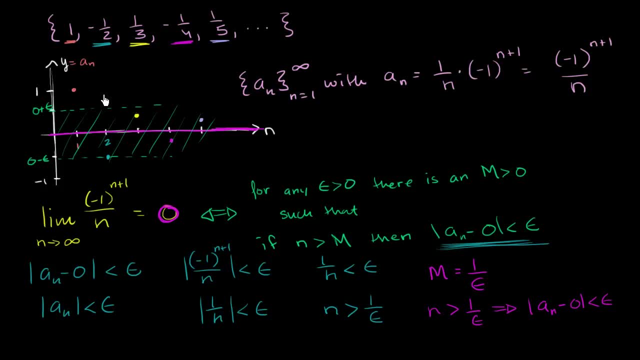 So as long as N is greater than 1 over 1 half, which is 2.. So in this case we could say: look, you gave me 1 half. My M is going to be a function of epsilon. It's going to be defined for any epsilon. you give me greater. 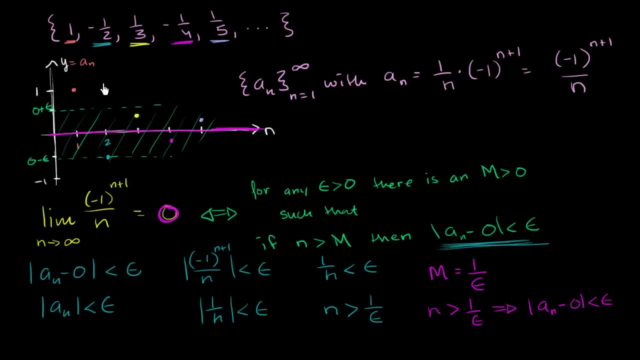 than 0. So here, 1 over 1 half is right over here. I'm going to make my M right over here And you see, it is indeed the case that my sequence is within the range as we pass for any N greater than 2.. 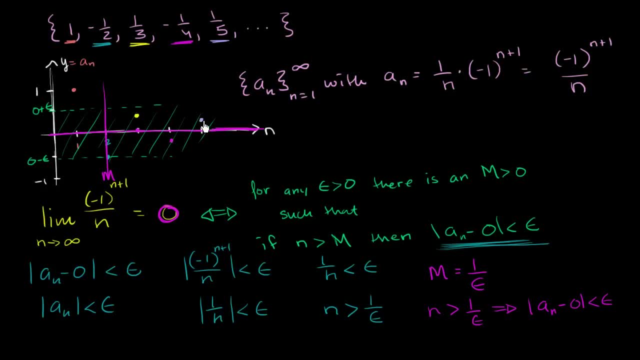 So for N is equal to 3, it's in the range For N is equal to 4, it's in the range For N equals 5.. And it keeps going and going, And we're not just taking our word for it. 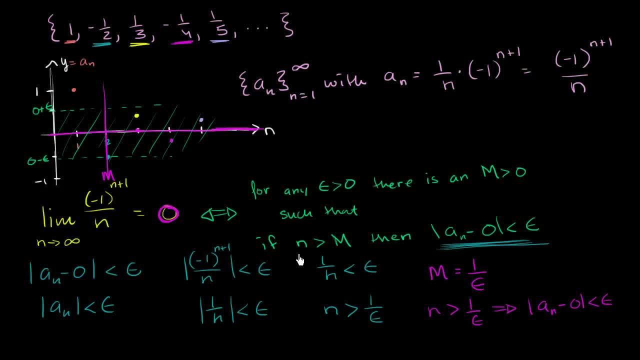 We've proven it right over here, So we've made the proof. You give me any epsilon I set: M is equal to 1 over that thing, And so for N greater than that, this is going to be true. So this is definitely the case.